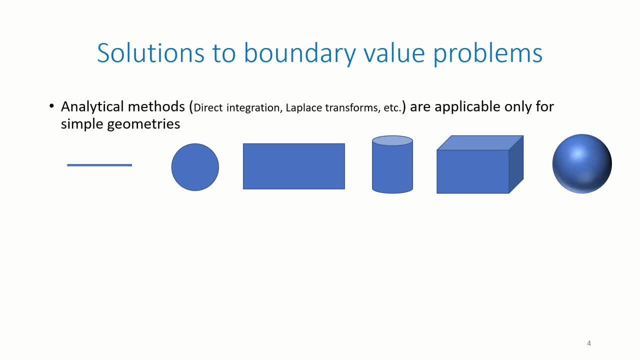 only for simple geometries as shown here. This stuff you might have studied in your undergraduate or graduate maths courses. Now the question is: how do we handle complex geometries, which are common in real world applications? And the answer is using numerical methods. 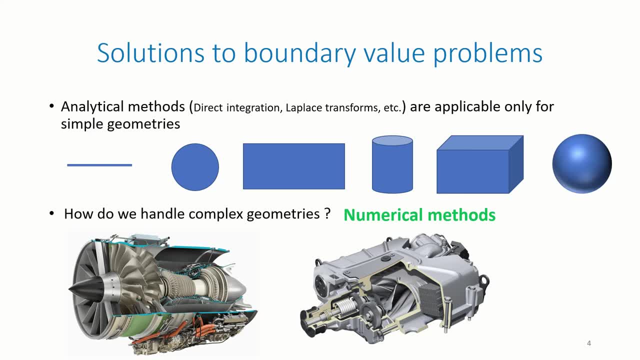 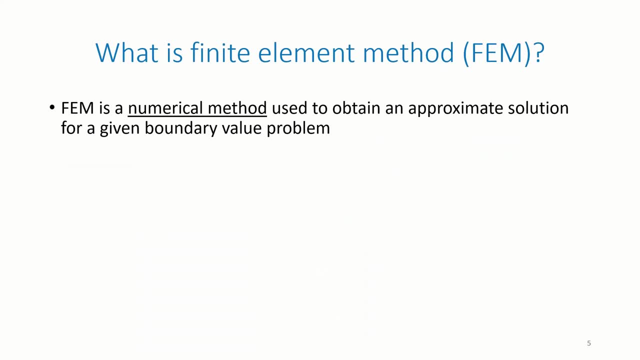 Okay now, what is FEM and how is it related to all these? You'll get your answers, don't worry. FEM is a numerical method which is used to obtain approximate solution for a given boundary value problem. This is what it does: It takes the boundary value problem and converts it into a linear. 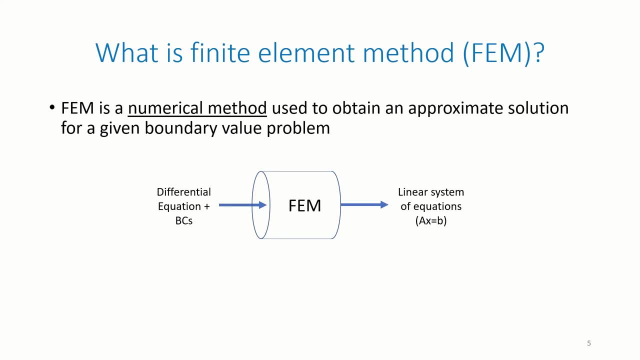 system of equations of the form ax equal to b. All those complicated equations you saw earlier will be converted into simpler forms And, as you know, ax equal to b could be easily solved using a computer. This is really important, and let me emphasize these two points again. 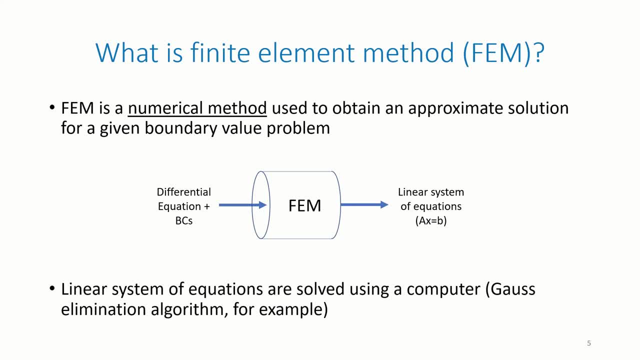 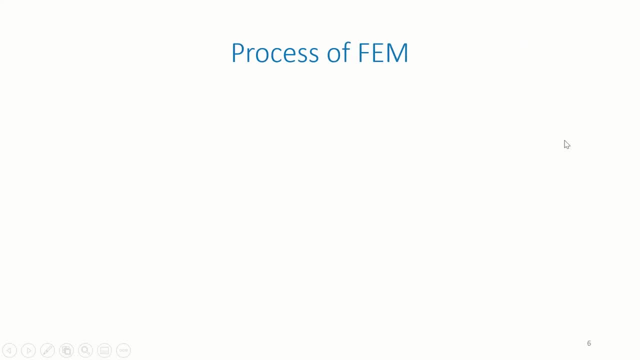 Number one: FEM is just a numerical method. Number two: FEM converts a boundary value problem into a linear system of equations. Keep this in mind. Let's look at the process of FEM, or learn how FEM works. To illustrate, I am taking 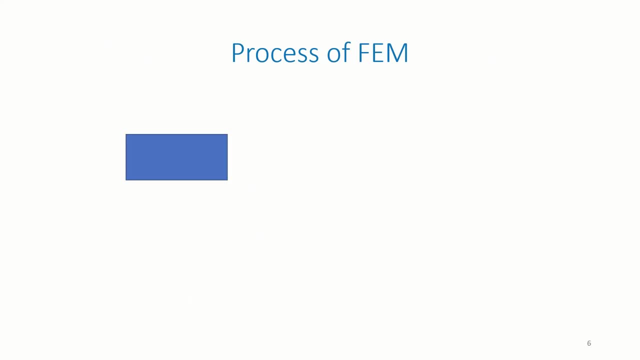 a rectangular plate as an example, But remember, this is applicable for any shape. Let me remind you that the objective here is to find the solution you had for the boundary value problem in this domain. In the first step, we divide our original geometry into smaller pieces. 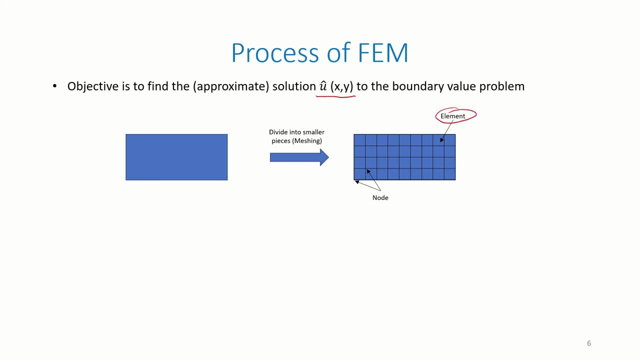 Each smaller piece is divided into smaller pieces. Each smaller piece is divided into smaller pieces. Each smaller piece is divided into smaller pieces. Each smaller piece is called the element, and all the intersection and corner points are called as the nodes. The process of dividing itself is called as meshing, and it is one of the key steps in FEM. 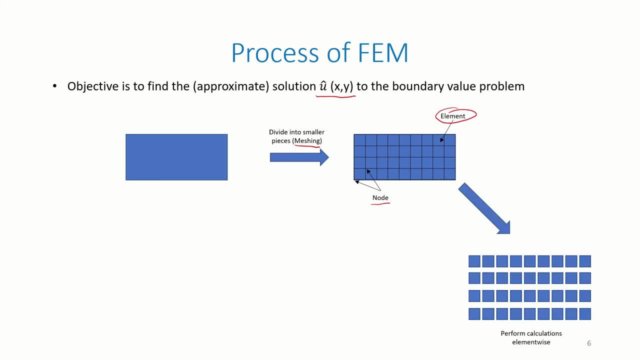 After meshing, we consider one element at a time and perform calculations. Likewise, we do our calculations on all the elements separately. Next, we assemble all this information together and we obtain the solution you had at all the nodes of the domain. Lastly, we do further calculations to obtain the field. 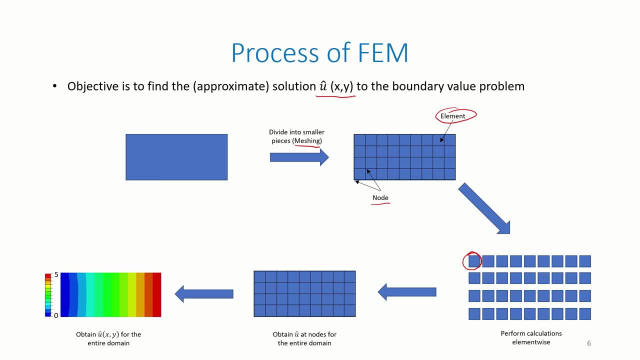 solution for the entire domain. That's the whole picture of a FEM in layman terms. Basically, it follows the divide and conquer process. However, the beauty of FEM lies in its mathematical treatment. Let me give you a flavor of it, without getting into finer details, so that you appreciate the FEM better. Let's 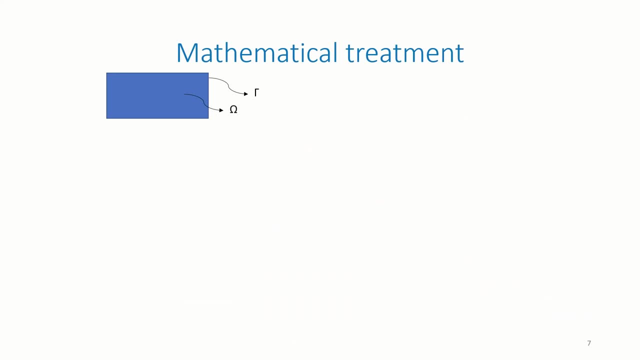 consider the same geometry as before, but here we divide this into two regions. The outer boundary is called as gamma and the inner region is omega, as shown To show the mathematics. I am taking a boundary value problem with the Poisson's equation, which is dou square u by dou x square, plus dou square u by dou y. 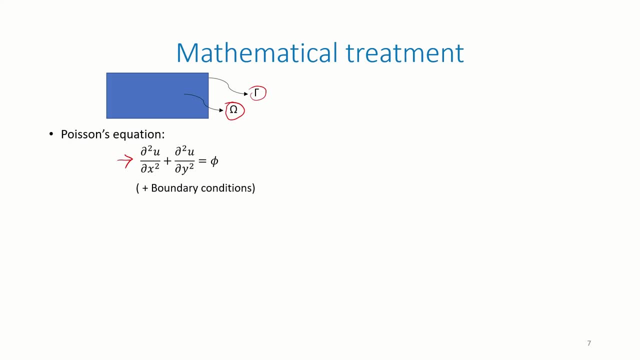 square equal to 5.. Of course, there are also boundary conditions associated with it, defined in gamma. If we consider u e as the exact solution, then it must satisfy this equation. If we consider u e as the exact solution, then it must. 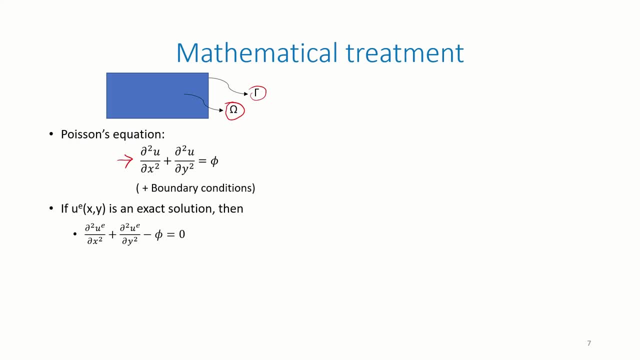 satisfy this equation. If we consider u e as the exact solution, then it must satisfy the above equation. so we will have: dou square u e by dou x square, plus dou square u e by dou y square minus 5 equals 0.. As I mentioned before it, 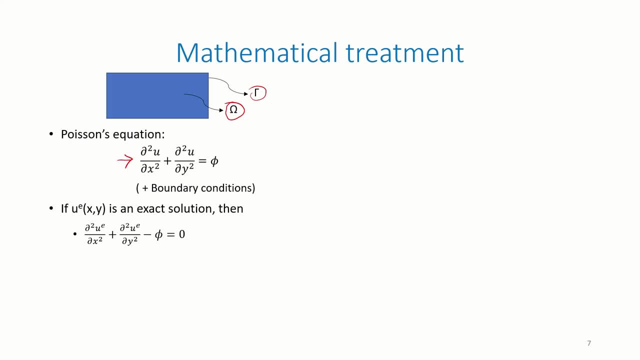 will be very difficult to obtain an exact solution for real-world problem. Instead, let's try to find an approximate solution. u hat, Since this is approximate, it will not exactly satisfy the Poisson equation. Hence we will have this term not equal to 0 and let's call this as the residual R To get a real 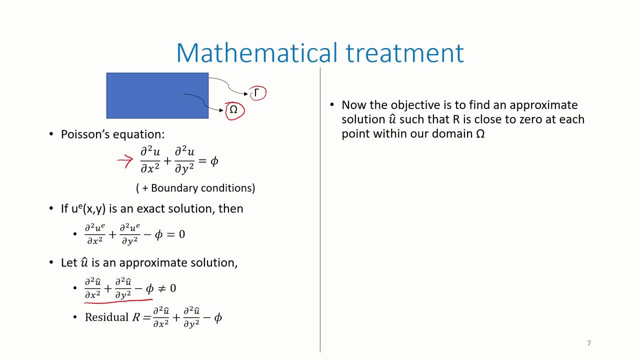 reasonable u-hat. we must try to make the value of r as close to zero as possible at each point in omega. So to make r close to zero we define what is known as the weighted residual statement. Here we integrate the product of the residual with a known weight. 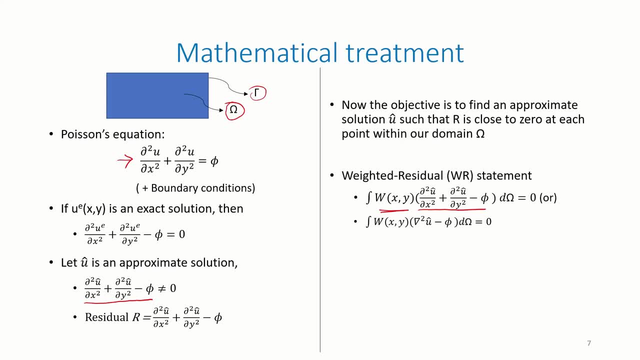 function w over the entire domain and set it equal to zero. In this equation I am just using the Laplacian operator del square instead of dou square by dou x square plus dou square by dou y square. Then if we integrate this equation by parts, we get the following equation: 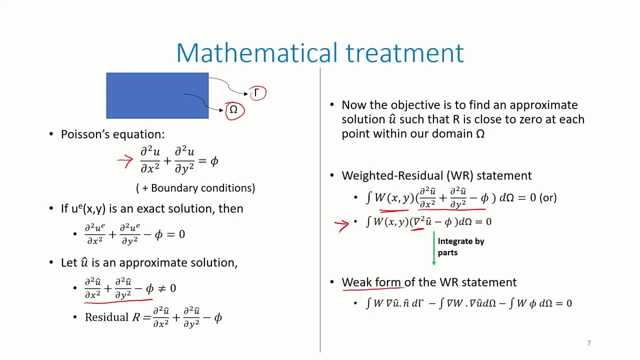 known as the weak form, And there is a reason it is known as the weak form and I would like you to explore that aspect. If you observe the weak form equation, we have this term in terms of d gamma, which is a boundary term and is related to our boundary conditions. 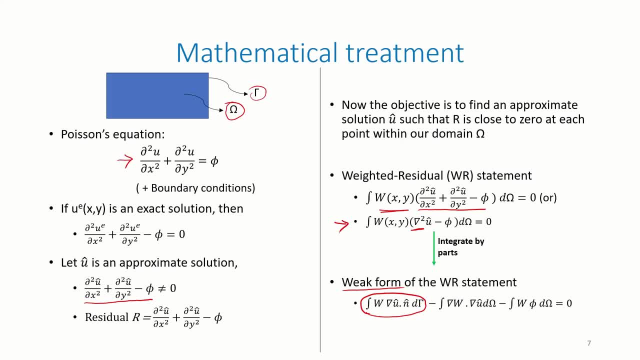 This weak form is a boundary term, So we have a boundary term of d gamma, which is related to our boundary conditions. This weak form is one of the significant steps in the FEM process and I would say this is where FEM starts. You may have two questions. 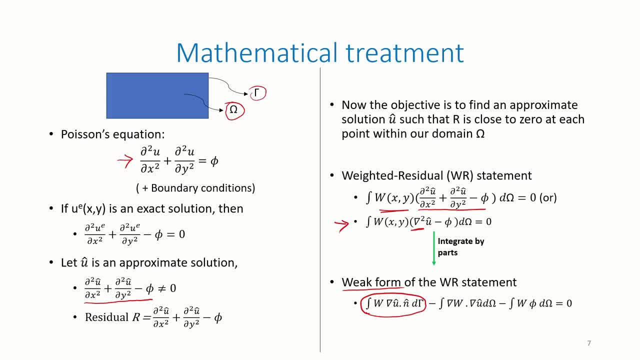 at this point. Number one, how does FEM convert the boundary value problem into linear system of equations? And number two, how all these equations fit into our process of FEM. These will be answered in the next slide. Just to remind you, we started with the boundary value problem and we ended with the weak form. 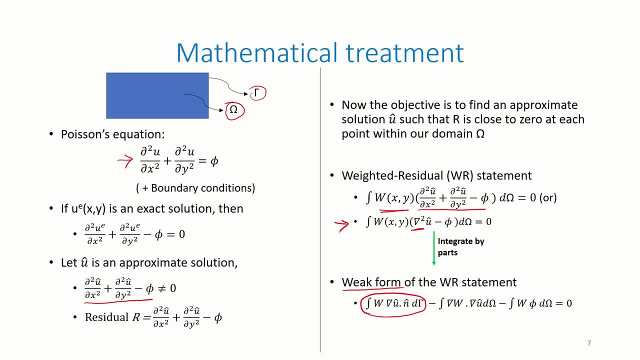 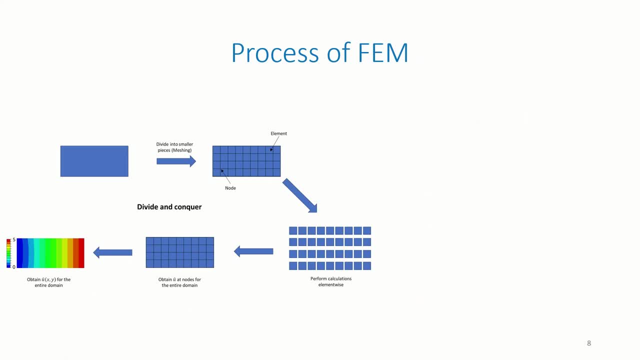 Let us move forward. We have discussed this process before. Let us try to see how the mathematics is associated with these steps. The weak form, as we saw, is defined for the entire domain. After we mesh, we define the weak form for each element and not for the 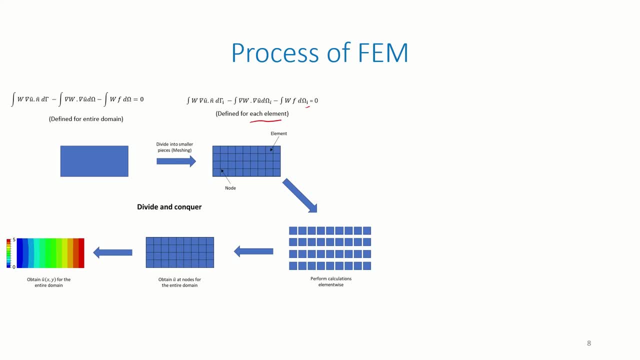 whole domain. I represents the ith element. Let us see what goes on in the element-wise calculations. This is where the magic happens. Let us isolate one element and see what is going on. The element here is a continuous domain. Imagine it is a collection of infinite points and our unknown u hat i is a field. 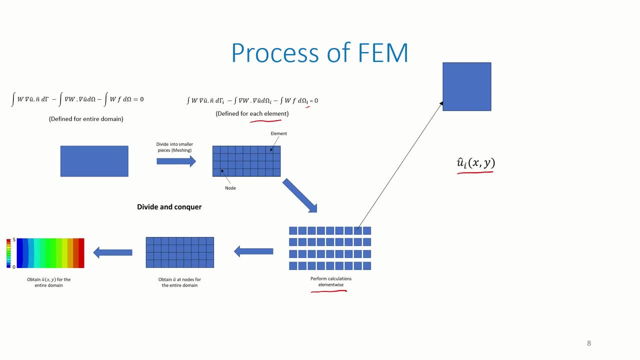 quantity or a function defined for this element. You know, finding a function is always a complicated task. Instead of having our unknown as a function, if we could have our unknown as an array of numbers, that would make our life much easier. Instead of u hat, x, comma y, we have u1 hat, u2 hat, u3 hat and u4 hat, defined at the respective 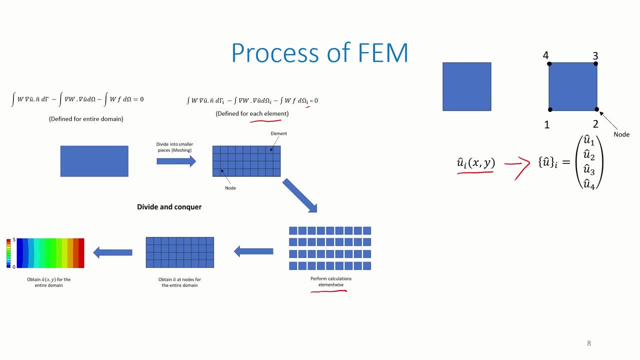 nodes of the element A function to just four numbers. Remember that This transformation is done by what we call as the piecewise interpolation and is given by the following equation: u hat equals n1, u1 plus n2, u2 plus n3, u3 plus n4, u4.. I personally believe that this is the 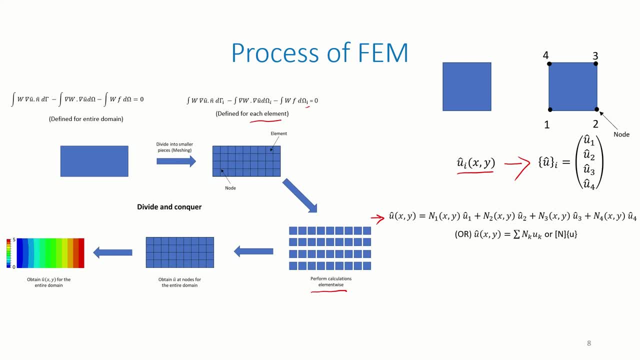 magic equation of FEM. n1, n2, n3, n4 are known as shape functions in FEM and, importantly, they are the known functions which depend on the shape of the element. So by this equation we are writing an unknown function. u hat, in terms of known functions, all your n1,, n2,. 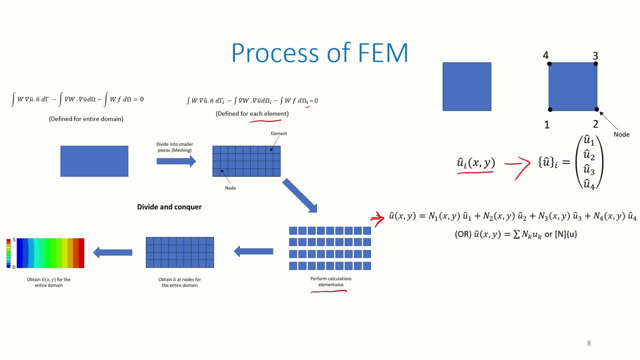 n3, n4 and unknown numbers, u1, hat, u2, hat, etc. We can also interpret this equation as a magic equation of FEM. Here's where the interesting part comes. If you substitute this u hat equation into the weak form and do some manipulations, you magically end up with a linear system of equations. 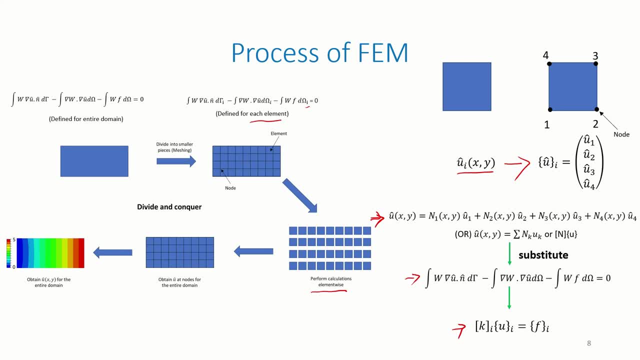 for that element. That's how FEM converts a boundary value problem into linear system of equations. And remember, this is just for one element. You need to do the same for each and every element. Here small k is called as the element stiffness matrix and small f vector in solid mechanics. 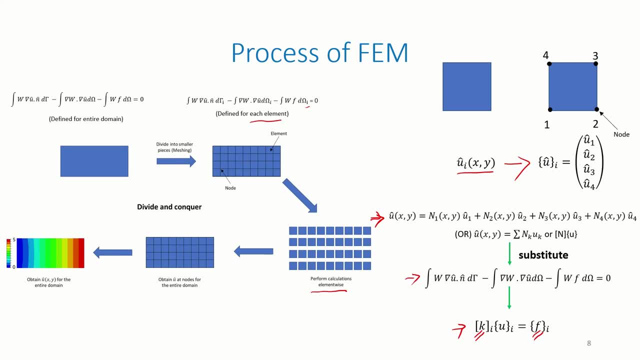 is called as the element loader force vector. The solution is not yet complete. Now you need to add together the contribution of all the elements. When you do that, you get a linear system of equations for the whole domain, as shown here. Capital K represents the global. 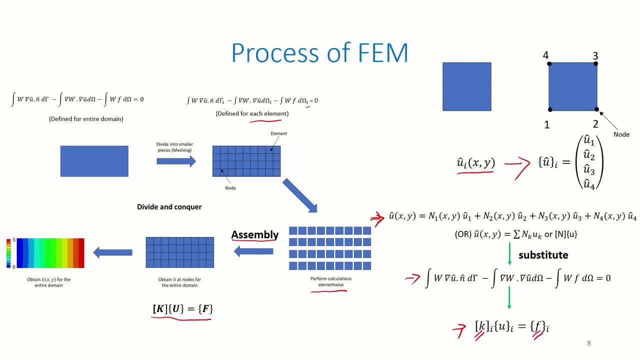 stiffness matrix. Capital F represents the global force vector and the number of equations will be equal to your number of nodes. By solving this equation we get u hat values at all the nodes in the domain. Then we could use the interpolation equation to obtain the field representation of u hat for the entire. 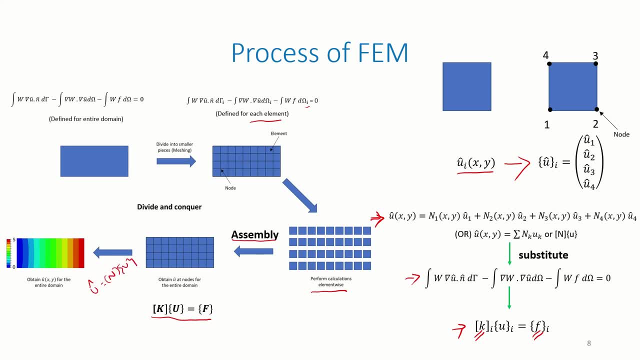 domain. Lastly, a common choice for the weight function w is the shape function n. When we do that, it is known as the Galerkin finite element method. That's why we use the Galerkin finite element method. That concludes the whole process of how FEM works. Let me take a step back and highlight 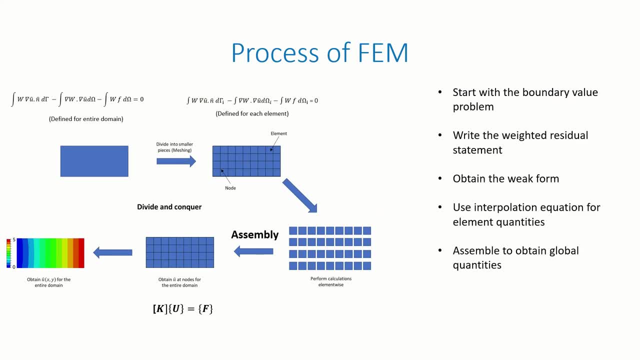 the important points. We start with the boundary value problem, Then we write the weighted residual statement, Then we obtain the weak form for each element. Later we use the interpolation equation to obtain the element level quantities. and then we do assembly and obtain the global.